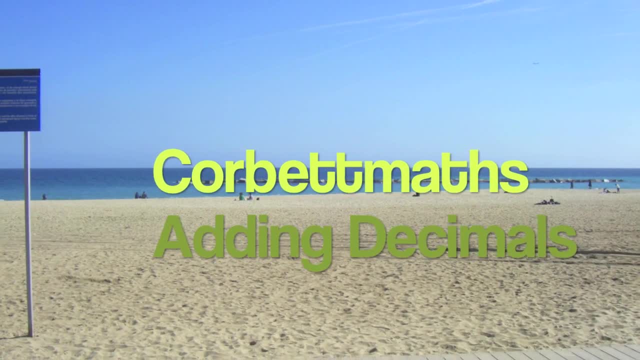 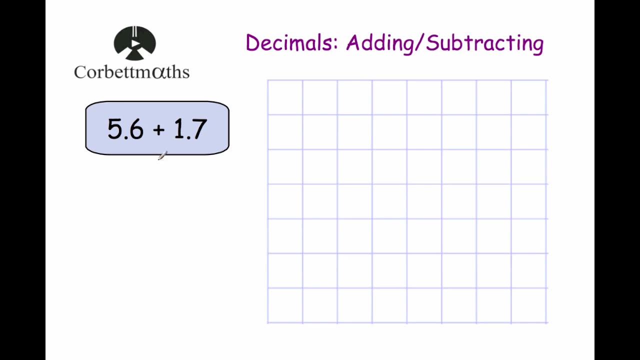 Hi and welcome to this Corporate Miles video on adding decimals and subtracting decimals. So let's have a look at a few examples. Our first example is 5.6 plus 1.7.. Now, if I was working at 5.6 plus 1.7, the first thing I would do is I would lay it out very carefully. 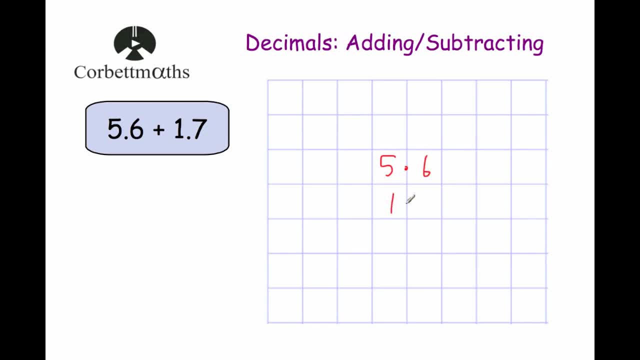 So I'd write 5.6 and 1.7, lining up the digits in the units column and lining up the digits in the tenths column, And I've also lined up the decimal points. Then I would put the line beneath it, like I would do in any addition, and I would put the plus sign, And also because 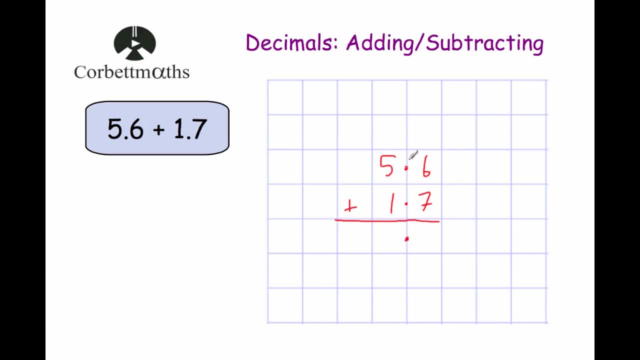 I've got the decimal points here. I'm going to put the decimal point there in the answer. So just lining up the decimal points, like so. And now I'm just going to work out the addition. So 6 plus 7 is 13.. So put the 3 down and carry the 1.. Now, in terms of the 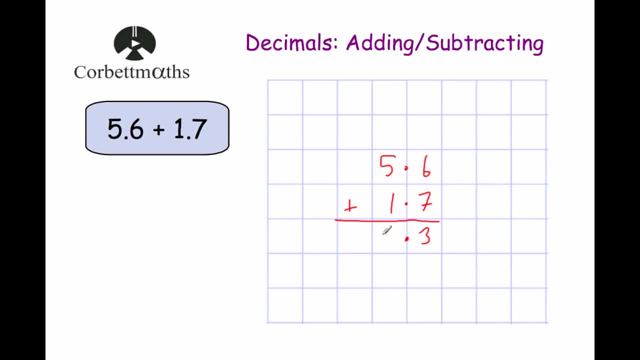 carrying. you might have a favourite place where you carry it to or where your teacher tells you to carry it to. I prefer carrying it here. the 1. Some people put it up here or down there. Just as long as you remember it, that's okay. So 5 plus 1 is 6, plus 1 is 7.. So our answer: 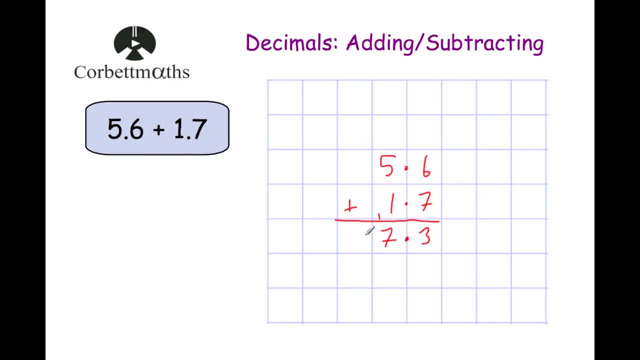 is 7.3.. So 5.6 plus 1.7 is 7.3.. Okay, our next example: Okay, this time we've got a subtraction, We've got 4.4 subtract 0.9.. So again, be very careful lining it out. So 4.4 subtract 0.9.. Again, lining up the 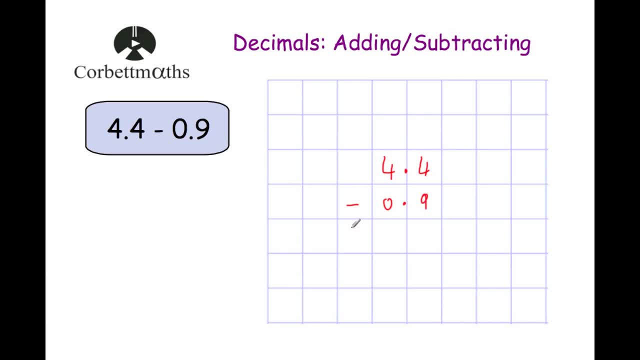 digits in the units column and in the tenths column And again put the line beneath it, because we're doing the subtraction And line up the decimal points. So we're going to put the decimal point there in the answer And then we're going to do our subtraction. 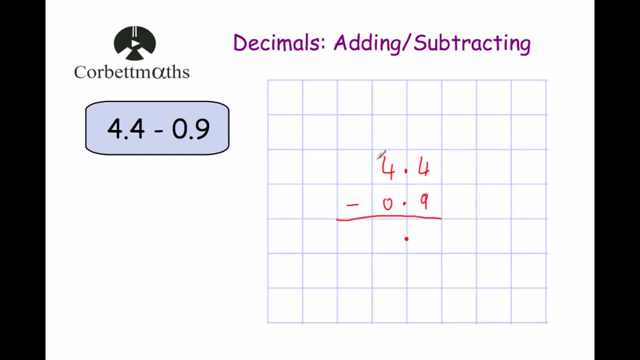 Okay, 4, take away 9.. We can't do So. we're going to borrow 1 from the units column, We're going to call that 3 and we'll carry the 1 over there to make 14.. Okay, 14, subtract 9. 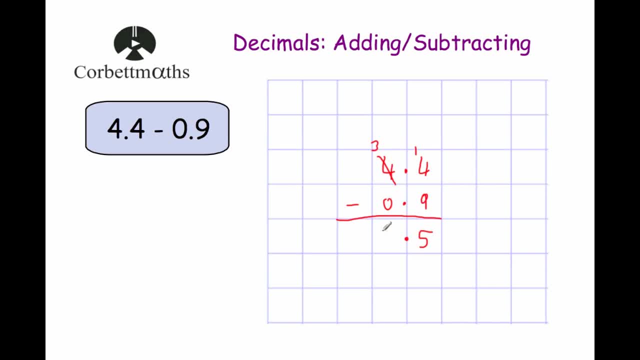 is 5.. So put the 5 there: 3 subtract 0 is 3.. So our answer is 3.5.. Okay, our next question. So our next question: we've now got 1.7 plus 3.5.. So we're going to do the subtraction. 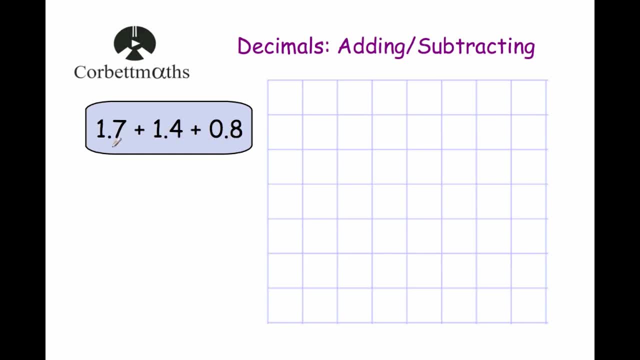 1.7 plus 1.4 plus 0.8.. So this time we've got three numbers we're adding together. It's just the same as before, but what we're going to do is we're just going to make sure we're. 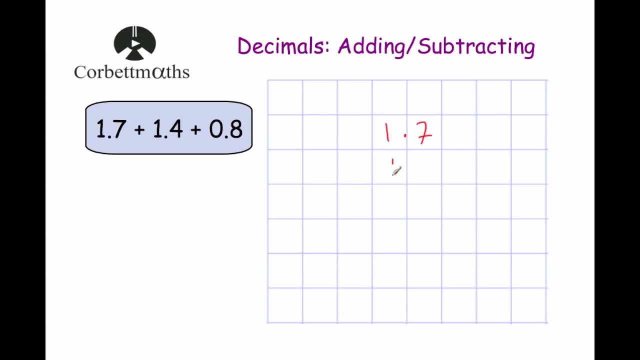 lining them all up, So 1.7, 1.4, 0.8.. Again, lining up the digits in the units column and the tenths column. We're lining up the decimal points and we're putting the line beneath. 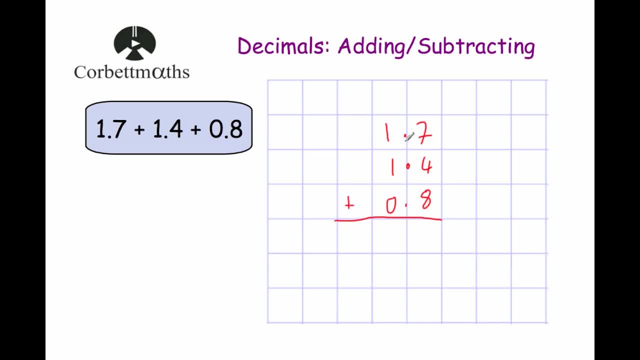 it like so And we put our plus sign Again, because our decimal points are here, our decimal points are going to be there in the answer, And then we just add: Let's do this one last time: 1 plus 7 plus 4 is 11, plus 8 is 19.. So put the 9 down and 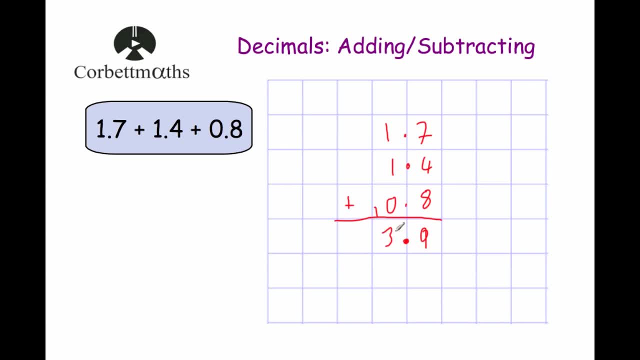 carry the 1.. 1 plus 1 plus 1 is 3.. So our answer is 3.9.. Okay, our next example Now. this one is a subtraction. Now you might notice that we've got 14 subtract 6.7.. So we're going. 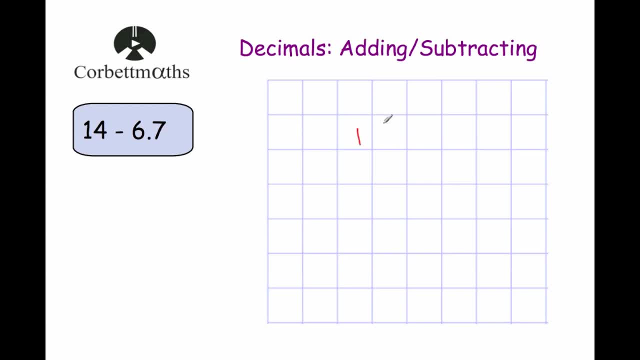 to be careful when we're lining these up. Okay, so we're going to write a 14 down. So we've got a 1 in the tens column and a 4 in the units column. Now our next number is 6.7.. So the units is 6 and we're going to add a 4 in the units column. Now we're going to add a 4.7.. We're going to add a 6.7.. So we're going to add 10s. So this one- here is the number. 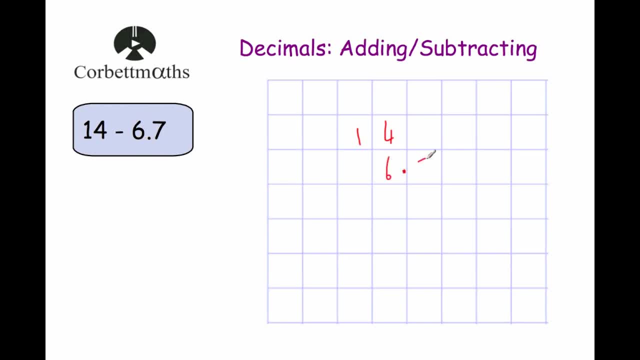 units is six, so we're gonna write six point seven. okay, so we've lined up the digits in the units column, the 14 has got a one. in the tens column we've got a decimal point here and then we've got this number. the six point seven has got. 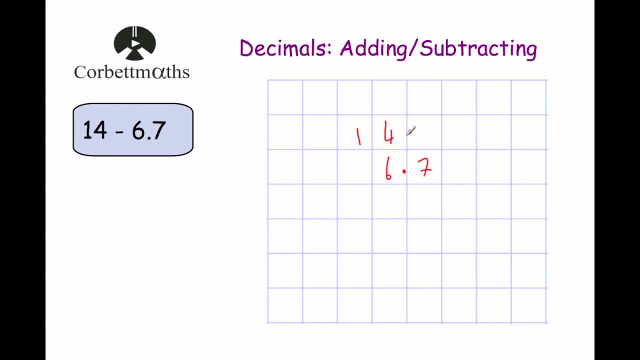 seven in the temps column. so what we're gonna do is we're gonna put a decimal point here in the 14 and we're gonna put a zero. it's very important, whenever you're adding, of adding or subtracting decimals, that they're the same length in. 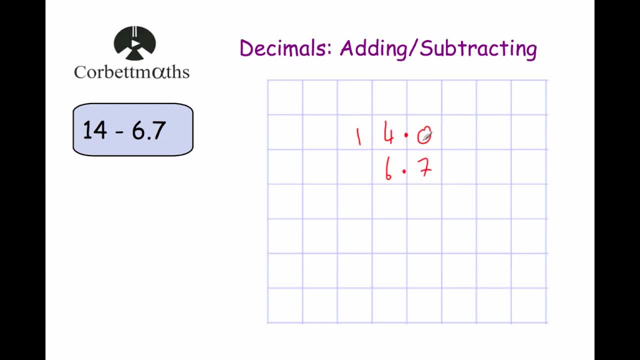 other words, if one of the numbers is good temps, that you put zeros in to make the other one have temps as well. if one of the numbers had hundredths, you add zeros to make the other one have hundredths as well. okay, the same length. that makes the question a lot easier. okay, so we're gonna put a line beneath. 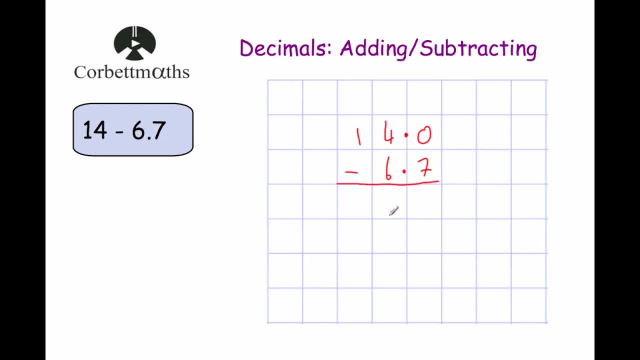 it, and then we're gonna put our subtraction sign and now we're just gonna subtract. so again, make sure we line up the decimal points. okay, zero take away seven. we can't do so, we're gonna need to borrow. so that's gonna be a comma three. I work, borrow and put the one there. ten take away seven is three. 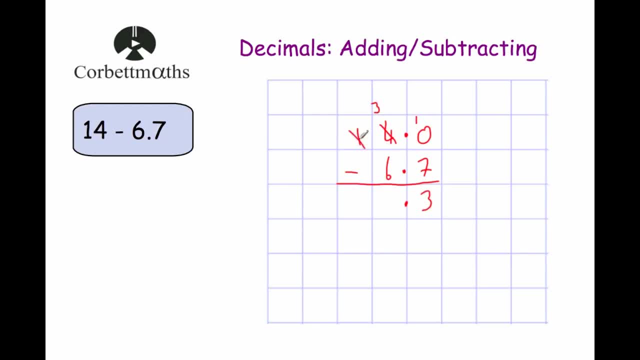 again: six. three take away seven is a comma, so it means one takes away seven. but there's no way you can six. we can't do so. we'll borrow, we'll call that zero and bring the one over there. 13, 13 take away six is seven. so answer is 7.3. so whenever you've got numbers that you're subtracting or adding, 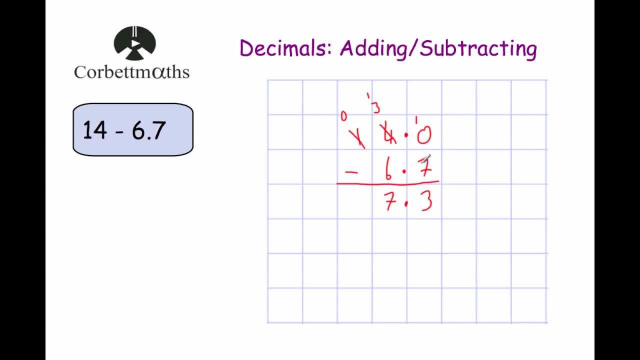 where one of them is slightly longer than the other. in other words, one might have tenths or hundreds or thousands. you add zeros to make sure that everyone's the same length, and also be careful whenever you're lining them up here. i was very careful to make sure that i put the units in. 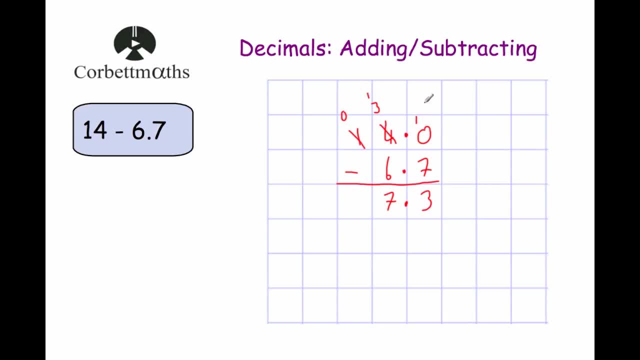 sort of one column, the tens, tens in another column, temps in another one, and so on. okay, our next example, okay, next example, is 0.78 plus 0.15. so again 0.78 and 0.15. again. i've been very careful. 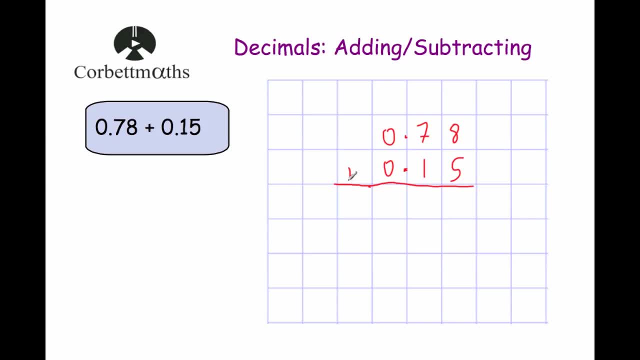 lining them up and i'll put the line underneath it and put the plus sign. so again, we've got a hundredths column, tenths column, units, column, and we've got our decimal points. so we'll put our decimal point here, so it's beneath the other ones, and we're going to add: so remember, starting from the right hand side. 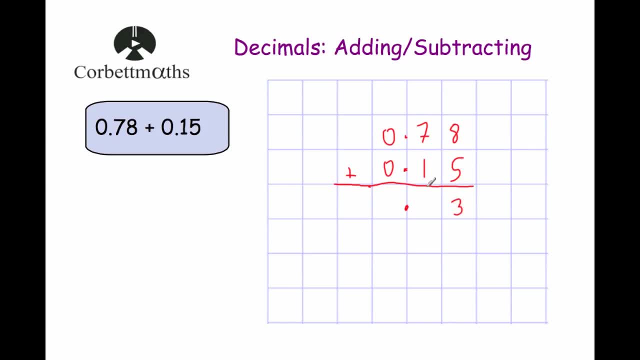 so 8 plus 5 is 13, put the 3 down, carry the 1, 7 plus 1 is 8 plus another one is 9, so answer is 0.93. okay, our next example, our next example is 8.25 plus 3.9. so again, be very careful when. 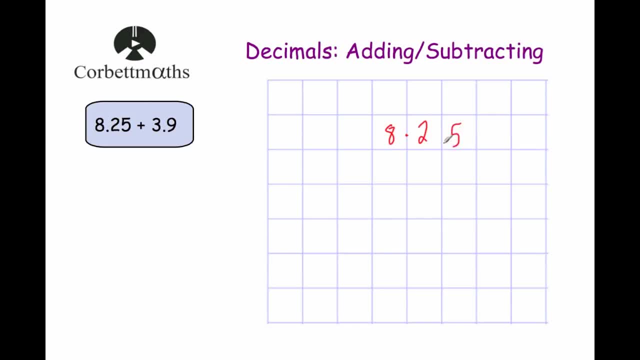 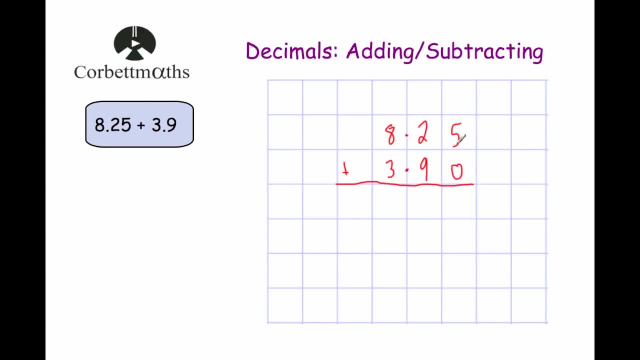 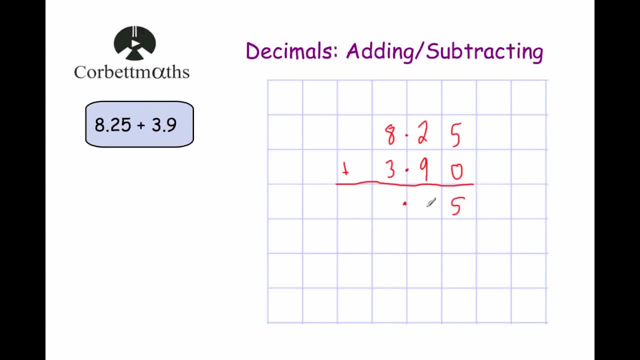 2. oh, you should get the decimal point. 2 plus 9 is 11, so put the 1 down and carry the 1. and 8 plus 3 is 11, plus 1 is 12, so we'll put our 12 down. so answer is 12.15. so let's have a look at our second.